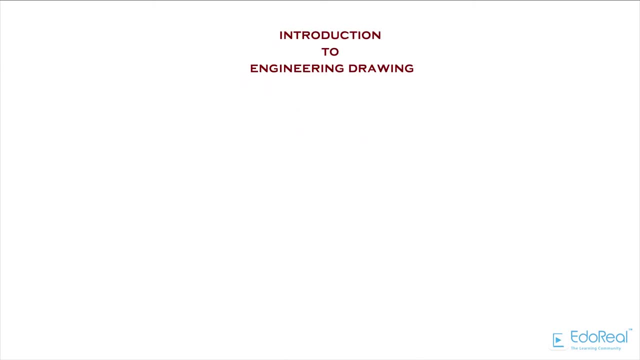 Introduction to Engineering Drawing. In this video, we will discuss Drawing, Engineering Drawing, Applications of Engineering Drawing, Instruments used in Engineering Drawing and different types of lines used in Engineering Drawing Drawing. Drawing is a graphical language that communicates ideas and information from one mind to another. 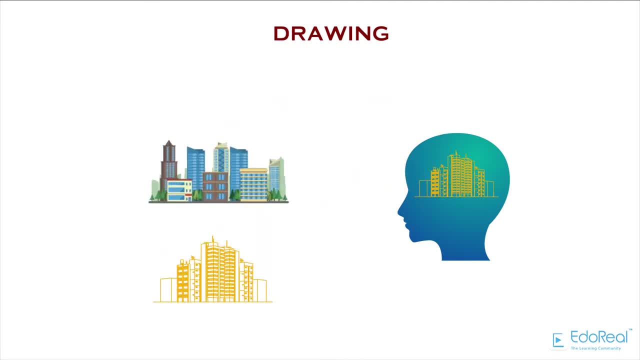 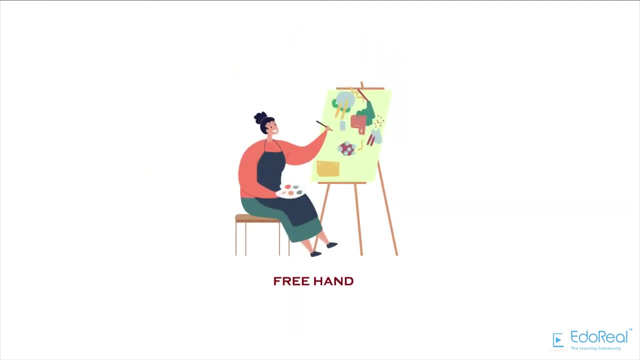 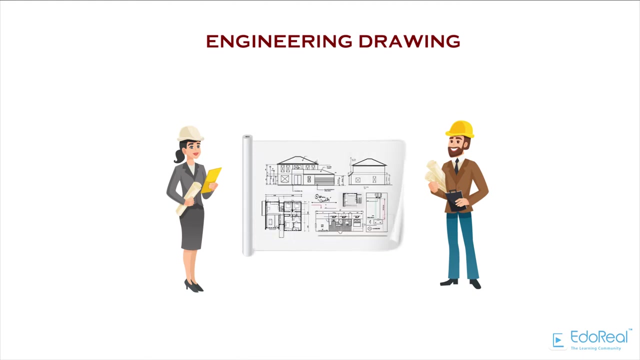 Or the graphical representation of any object or idea, can be termed as drawing. A drawing can be prepared either using a free hand or using engineering instruments, or using a computer program. Engineering Drawing- An engineering drawing- is a type of technical drawing used to fully and clearly define requirements. 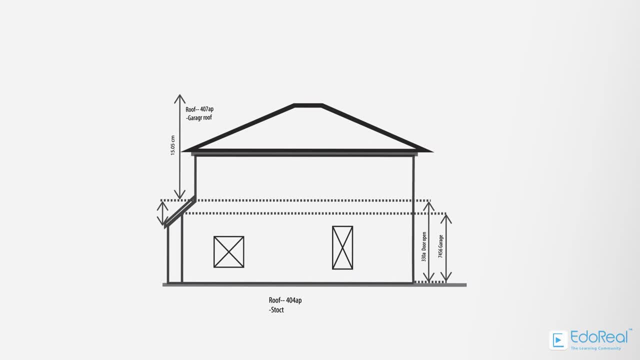 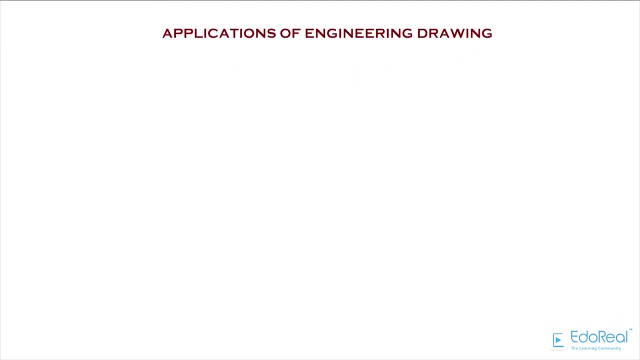 and capture all the geometric features of a product, such as dimensions for engineering. Drawing can be used in engineering products. Applications of Engineering Drawing. Drawing is used in manufacturing of all automobiles. Drawing is used in constructions. Drawing plays a vital role in engineering and it is essential to our daily life. 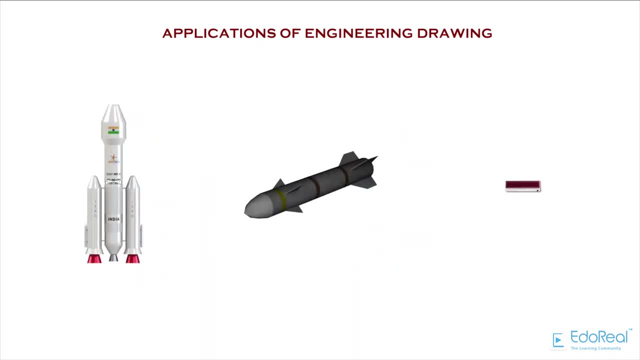 For example, construction of rockets, missiles, ACs, etc. initially they should need drawing to come out as a final output. Instruments are used in engineering. Instruments are used in engineering. Instruments are used in engineering. used in engineering drawing. Drawing board. Drawing sheet. Mini drafter- T-square Compass. 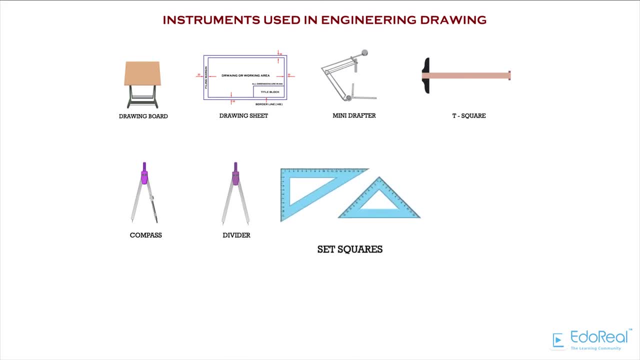 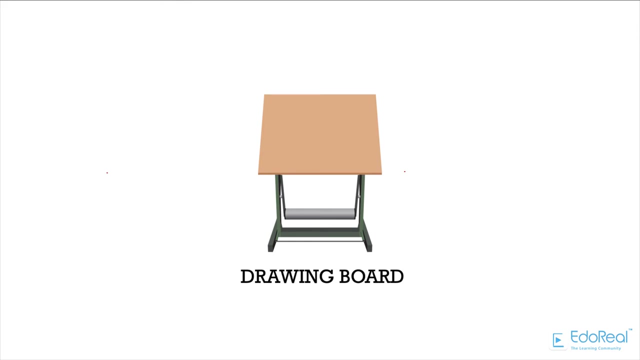 Divider, Set squares, Protractor, French curves, Pencils, Eraser. Let us describe each and every drawing instrument in detail: Drawing board. Drawing board is generally made of softwood and it is in a rectangular shape. It is used to support the drawing sheet, so the size of the board. 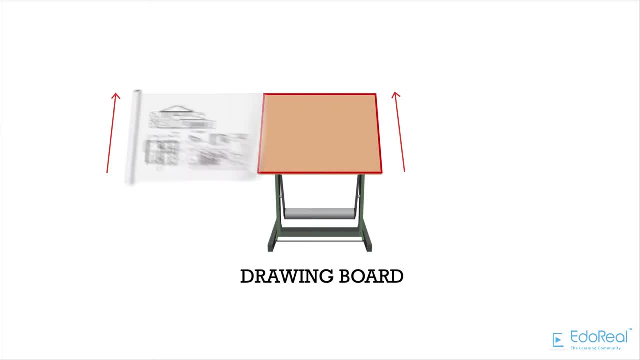 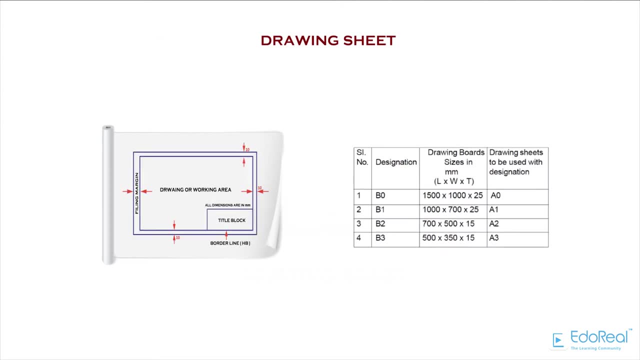 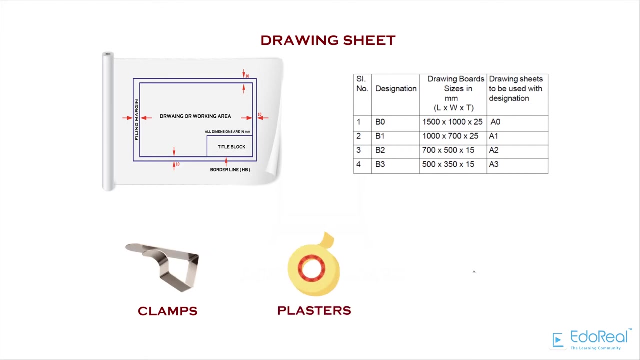 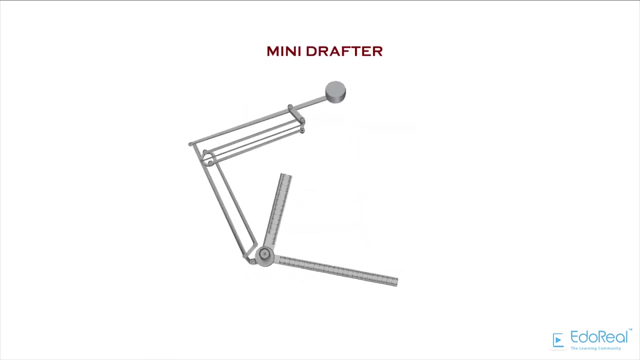 is made according to the size of the drawing sheet. Drawing sheet. Drawing sheet is a white paper on which an object is drawn, which is available in various sizes. To fix the drawing sheet to the board, clamps, Plasters, Paper holders are used. Mini drafter: Mini drafter is an instrument used for multiple 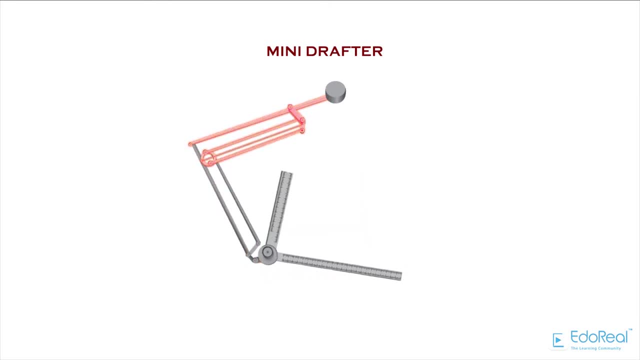 functions in drawing. It contains two arms which are adjustable to required angle, and at the end of the lower arm a scale set is attached. This instrument is fixed to the drawing board at one edge with the help of screw provided for the drafter T-square. T-square is used to fix the 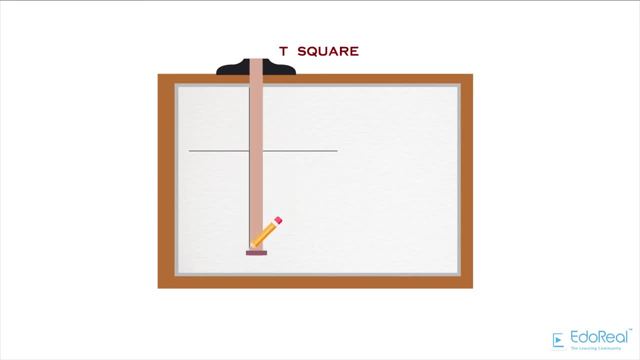 drawing sheet Drawing board. Drawing board is used to draw horizontal and vertical lines on a drawing sheet. The edge of the head is in uniform level and attached to the edge of the board. The working edge is used to draw lines anywhere on the sheet by moving the 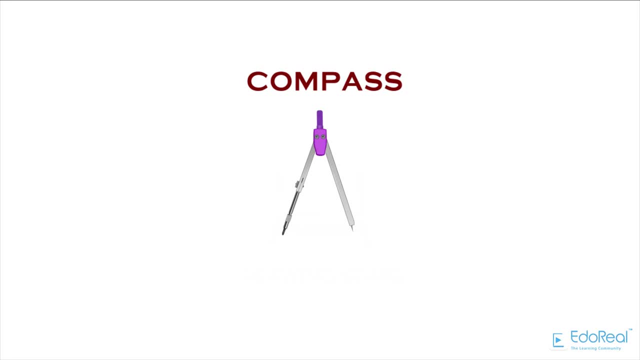 instrument: top to bottom: Compass. Compass is used to draw an arc or circle with known dimensions. on engineering drawing Divider. The divider looks like a compass but it is not a compass. but the difference is the two legs of the divider are provided with needles. 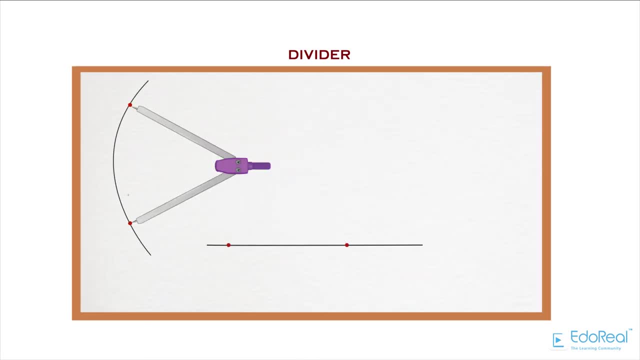 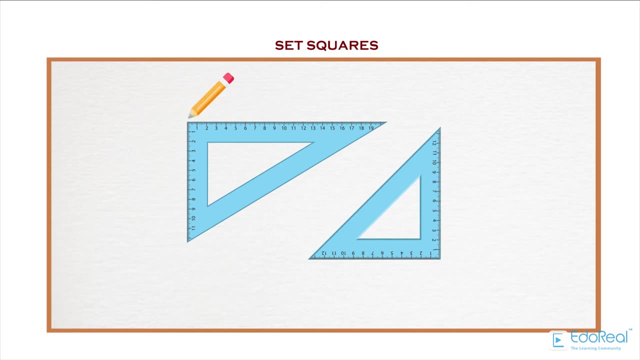 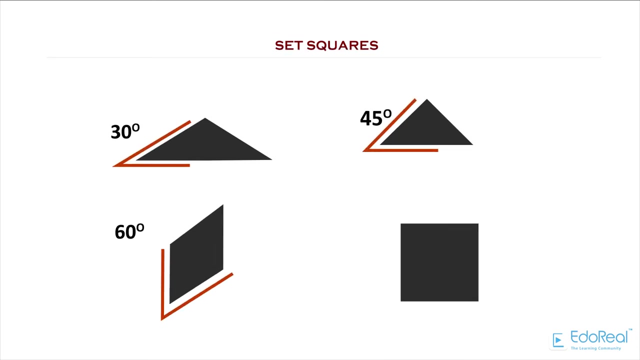 This is used to divide a line or curve into equal parts. It is also used to check the measurements Set squares. Set squares are used to draw lines with an angle between them In most of the structures. 30,, 45,, 60 and 90 degree lines are most common, So set squares. 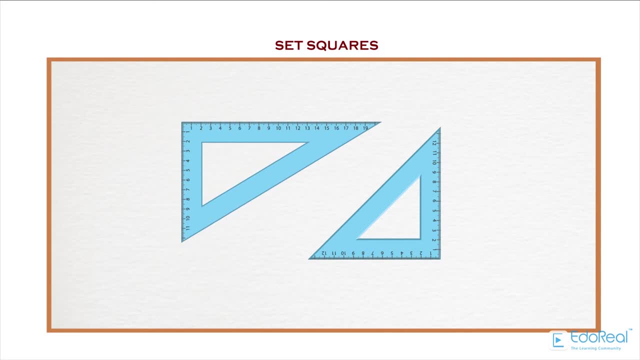 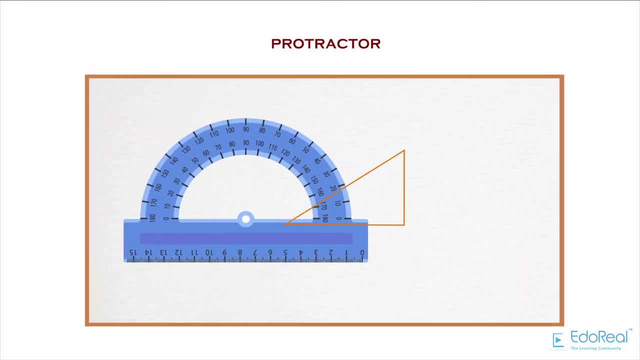 make the work easier for this type of drawing. Generally set squares are of 2 types. One is a 45 degree set square and another one is a 30 to 60 degree set square. Protractor. Protractor is used to draw and measure the. 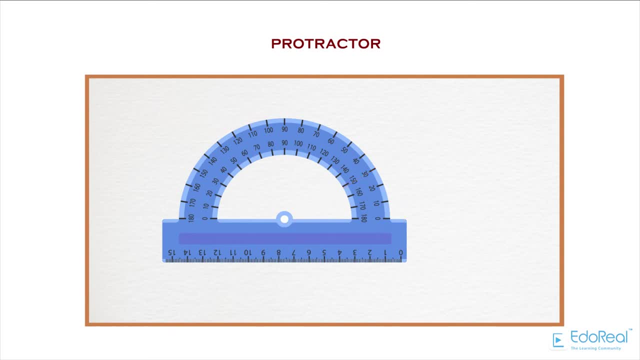 angles of lines in the drawing. It is in the shape of a semicircle and the edge of the semicircle part consists of reading with 1 degree accuracy. The bottom line joins the 0 degree to the 1200 degree line. The bottom line joins the 0 degree to the 120 degree. 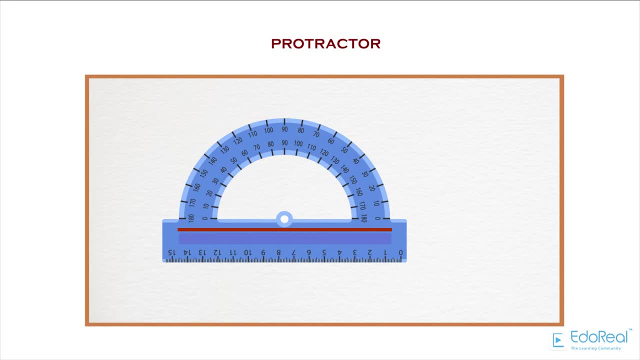 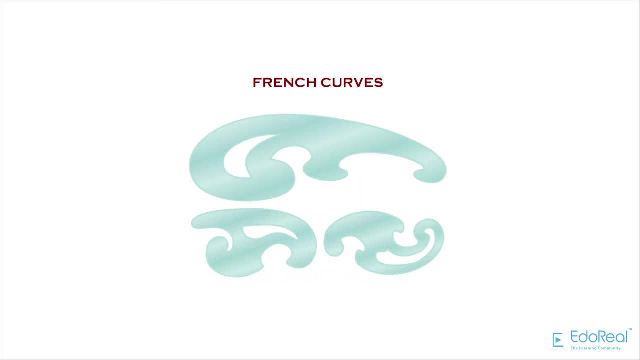 line. The bottom line joins the 60 degree line and the 240 degree line. The bottom line 180 degree. The center of this bottom line is marked as O or C, from which the angles are measured. French curves: French curves are made of plastic and they have irregular shapes. 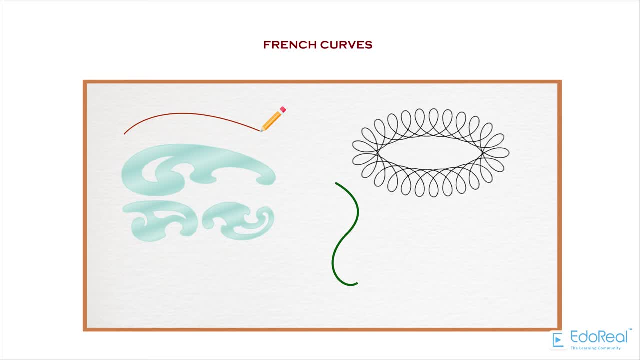 Sometimes the drawing requires irregular curves or shapes or arcs which cannot be drawn using compass. In that case, French curves are suitable Pencils: Pencil is used to draw on paper. Any type of pencil is not suitable for drawing. There are some limitations. The drawing appearance. 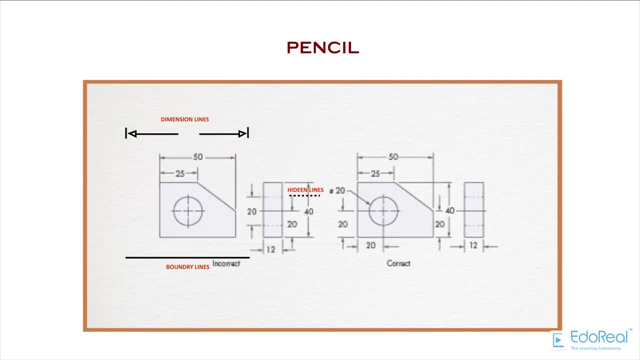 should be very neat and understandable. Every line of the drawing should indicate its importance. The following pencils are used in engineering drawings: 3H pencil. 2H pencil. 3H pencil. 3H pencil. 3HB pencil. 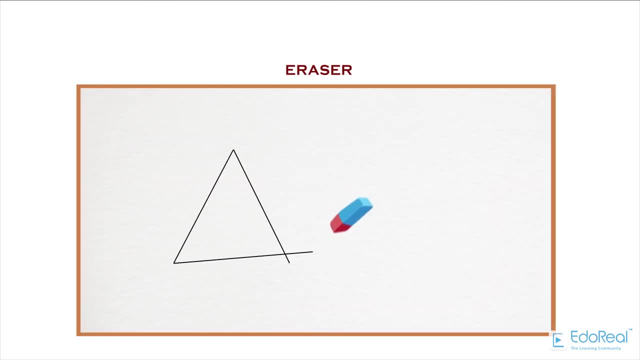 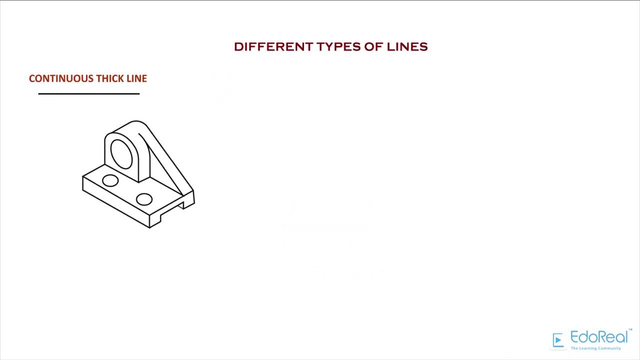 Eraser. Eraser is used to remove the lines or spots which are drawn by mistake or with wrong measurements. Next, we will see different types of lines used in drawing to indicate different parts of an object. Continuous thick line: This line is used to display outlines. 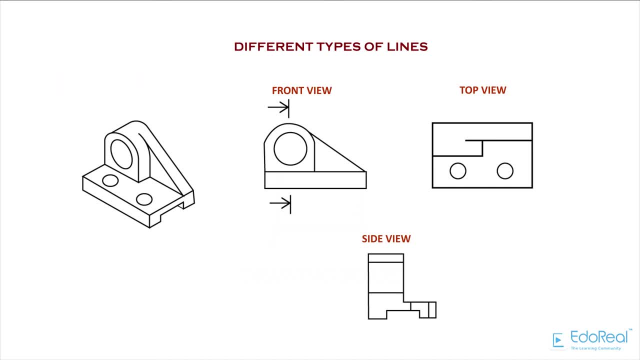 This line, Union line line and edges of the main drawing. Continuous thin line: This line is used for extensions, dimensions, projections, hatching leader, etc. Continuous thin free hand line: This line is used to show short break, irregular boundaries. 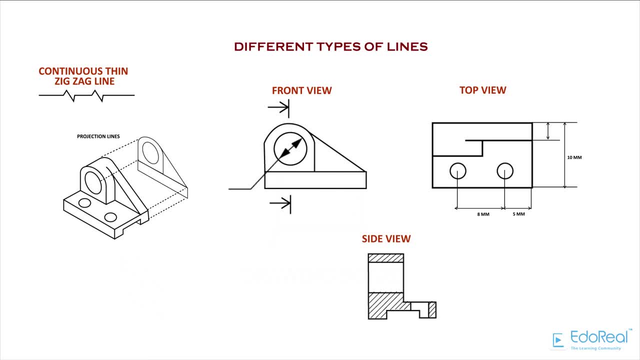 This line for stone: Mesquite, from Ruiz's Tunnel, Thin line with zigzags. Master piece, lame Car. relevant tools, forgartenscom. Water packed lines. This line is used to show a long break Dash line. This line is used to show hidden edges of the main object. 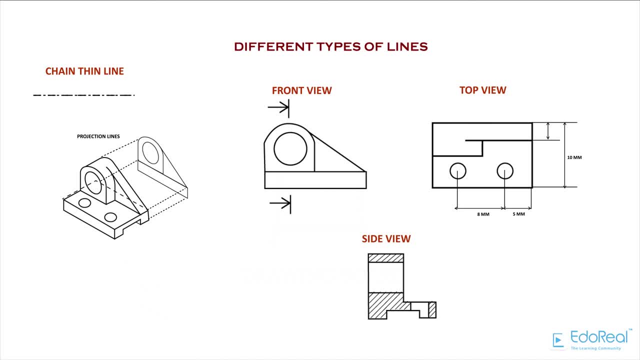 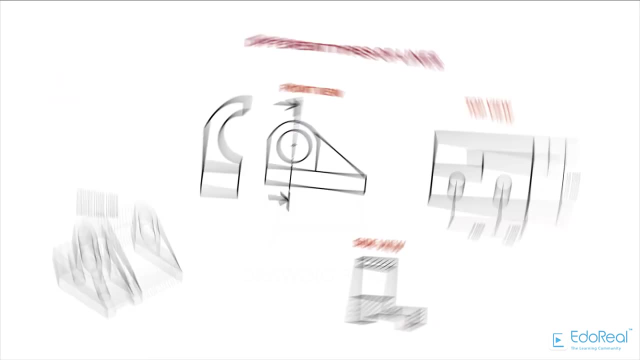 Chain thin line. This line is used to represent central lines for circles and arcs. Chain thin line with thick at the ends. This line is used to represent the location of a cutting plane. In this video, we have discussed the introduction to engineering drawing. 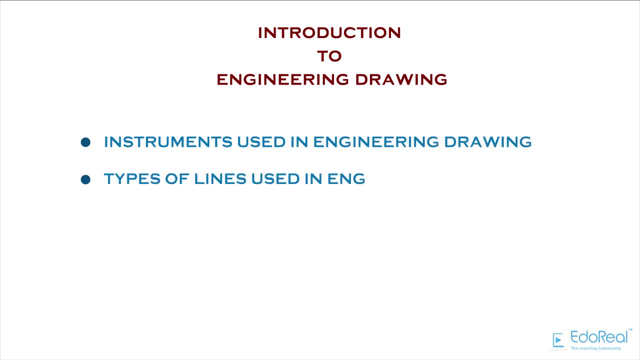 instruments used in engineering drawing. types of lines used in engineering drawing.